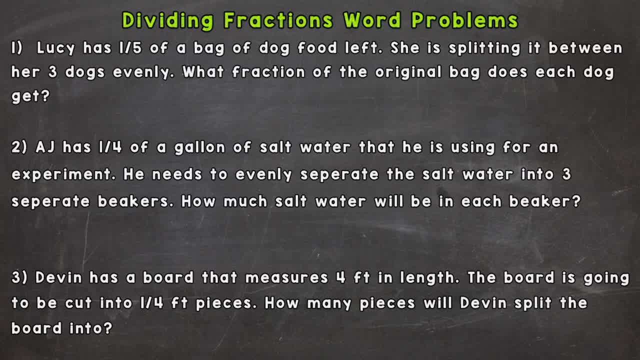 at number one here. Lucy has one-fifth of a bag of dog food left. She is splitting it between her three dogs. evenly. What fraction of the original bag does each dog get? Well, we're splitting something up or separating into groups. So whenever we're splitting or separating into 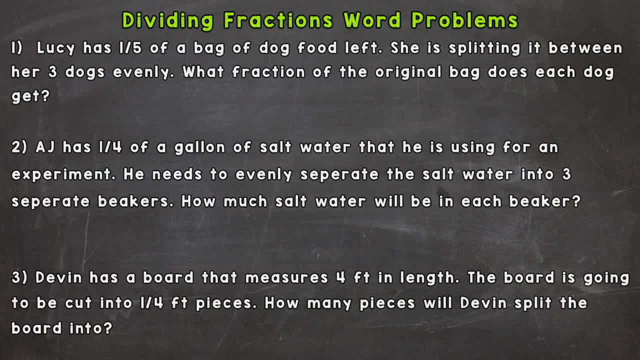 equal groups. we're going to use division Now. division orders us to divide into groups. So we're going to use division Now. division orders us to matters. so whatever you're splitting up, whatever objects being split up, needs to come first in your problem. so let's think: here we have 1, 5th of a bag of dog. 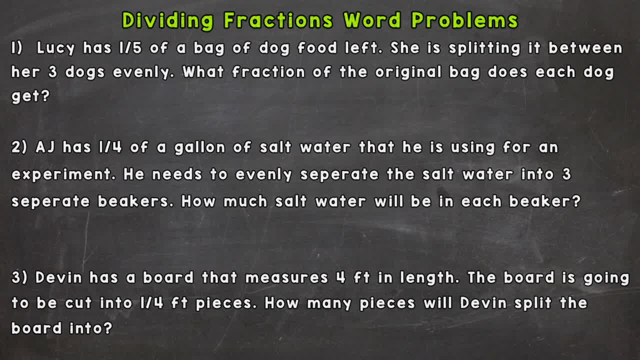 food. or we have three dogs, which object thing, person, animal, whatever the case may be, what is being split up in this problem? well, the dog foods being split up, so that needs to come first. so we need to do 1, 5th divided by, and how many? 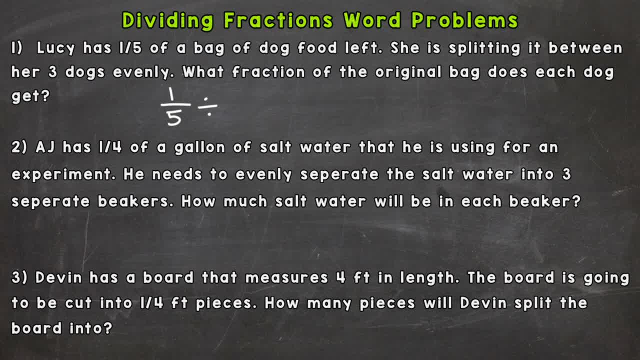 groups. are we splitting the 1, 5th of dog food into? well, there's three dogs, so that would be three groups there, so 1 5th of a bag of dog food split or divided between three dogs. so now we can keep switch and flip in order to solve. 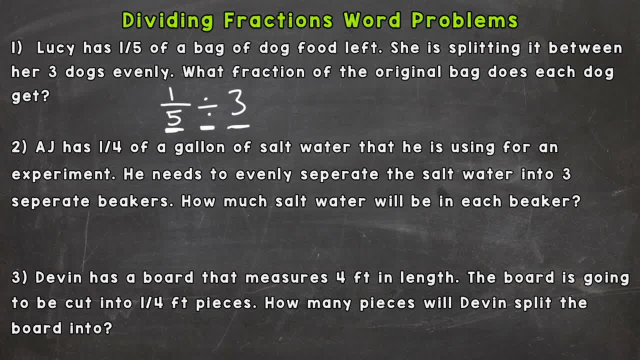 this now. I usually like to rewrite the problem underneath the division problem, but due to space here, I will write it to the right. so keep switch and we need to flip that 3 and it will now be 1- 3rd. now we can go straight across and get to our solution. 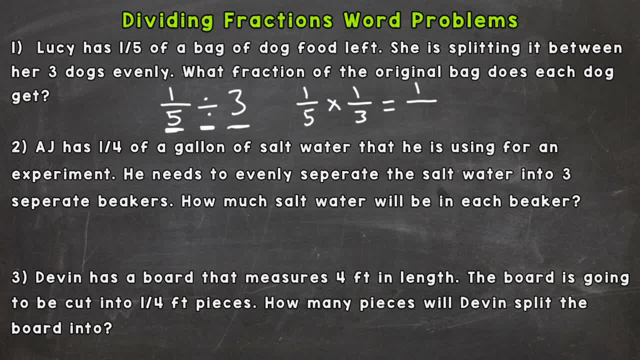 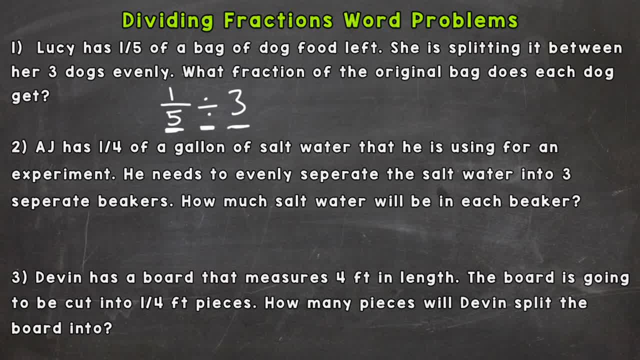 divided between three dogs, so now we can keep, switch and flip in order to solve this now. I usually like to rewrite the problem underneath the division problem, but due to space here, I will write it to the right. so keep switch and we need to flip that. 3. 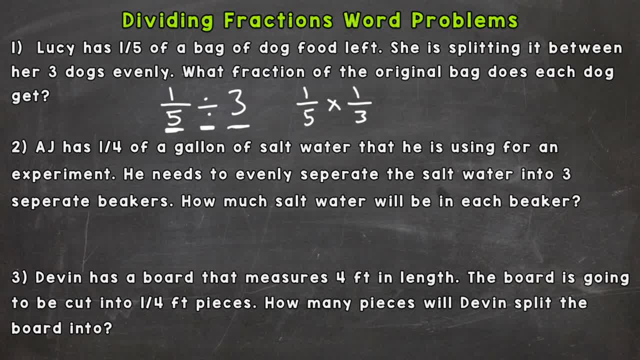 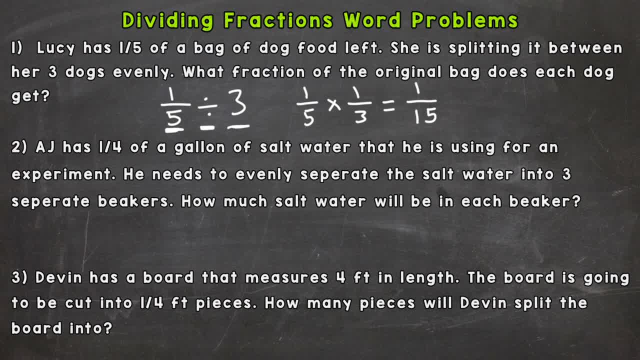 15th of that original bag of dog food. so 1, 15th of the bag, all right. number 2: AJ has 1, 4th of a gallon of salt water that he is using for an experiment. he needs to evenly separate the salt water into three separate beakers. how much salt? 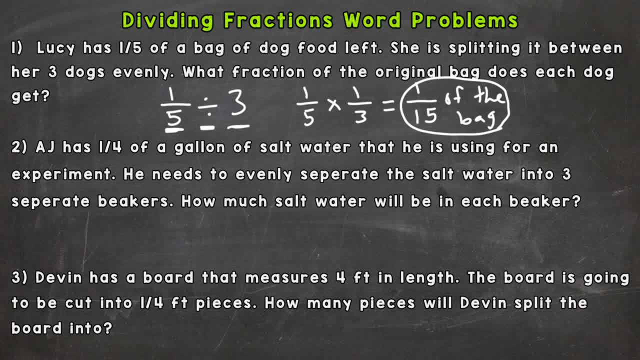 water will be in each beaker, alright, so we're separating into groups. so this is division again. and obviously all these problems on your screen are. but when everything's mixed together- add, subtract, multiply and divide- we need to know what type of situation will use division. and here we're separating into groups, so we 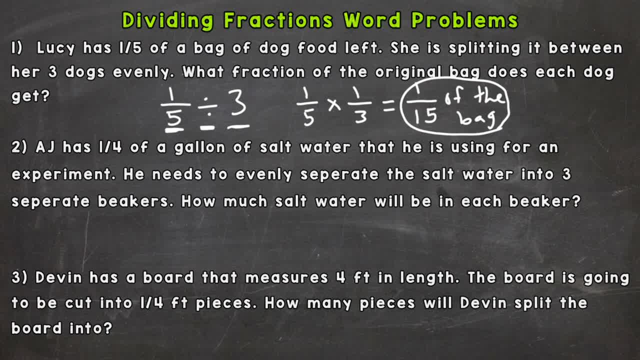 need to think what is being separated and the salt water is. so we have 1, 4th of a gallon and we're dividing it or splitting it between three separate beakers. so here, 1 4th divided by 3, keep, switch and flip. now we can go straight. 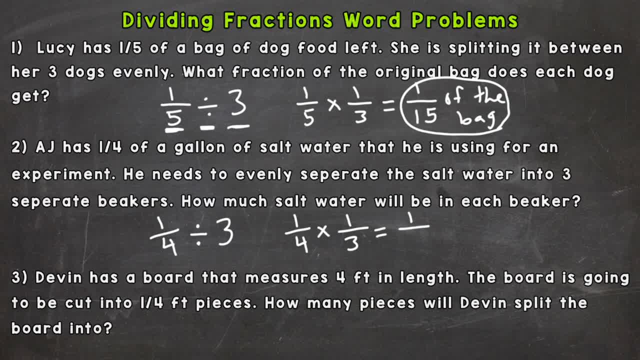 straight across. 1 times 1 is 1. 4 times 3 is 12. so each beaker has its own beaker is going to get one-twelfth of a gallon, Alright. lastly, number three, Devin has a board that measures four feet in length. 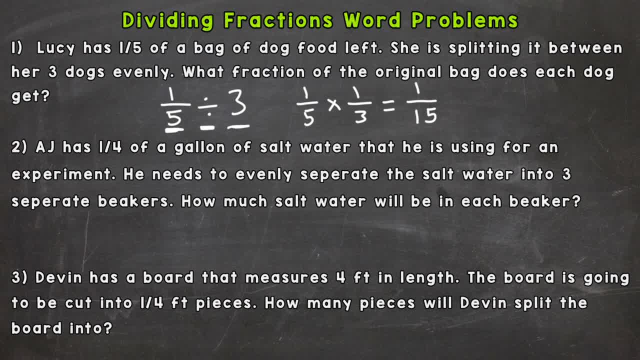 15th of that original bag of dog food. so 1, 15th of the bag, all right. number 2: AJ has 1, 4th of a gallon of salt water that he is using for an experiment. he needs to evenly separate the salt water into three separate beakers. how much salt? 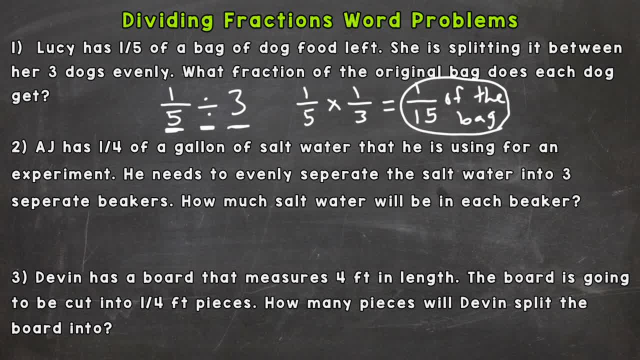 water will be in each beaker, alright, so we're separating into groups. so this is division again. and obviously all these problems on your screen are. but when everything's mixed together- add, subtract, multiply and divide- we need to know what type of situation we'll use: division, and here we're separating into groups, so we 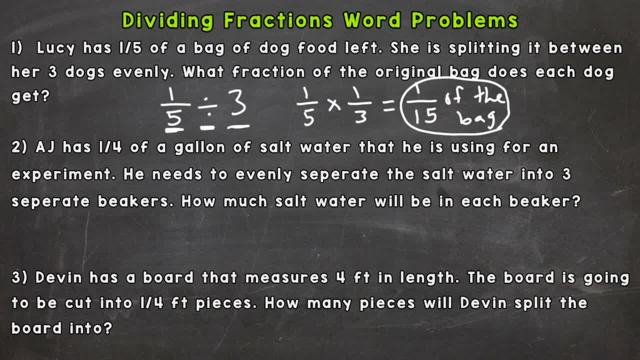 need to think what is being separated and the salt water is. so we have 1, 4th of a gallon and we're dividing it. we're splitting it between three separate beakers. so here, 1 4th divided by 3, keep, switch and flip. now we can go straight. 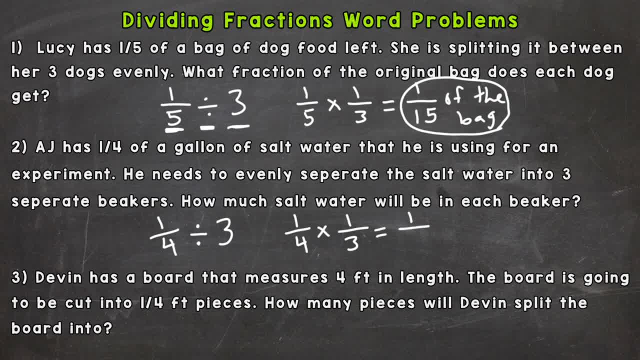 straight across. 1 times 1 is 1. 4 times 3 is 12. so each beaker is going to get 1, 12th of a gallon. all right. lastly, number three, Devon has a board that measures 4 feet in length. the board is going to be cut into 1, 4th of a foot piece. 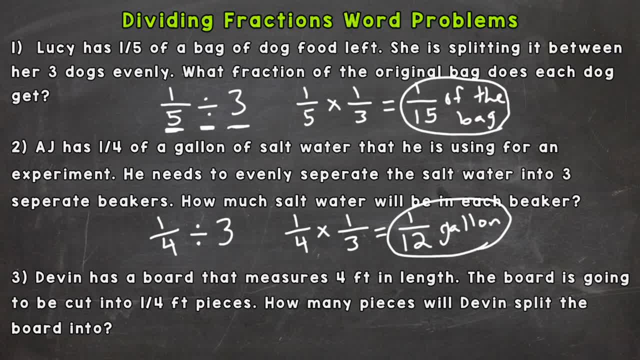 is 1- 4th of a foot pieces. how many pieces will Devon split the board into? so we're starting with 4 feet and we're splitting that 4 feet into groups of a fourth right. so we are dividing 4 by 1- 4th. what are we splitting up? well, the 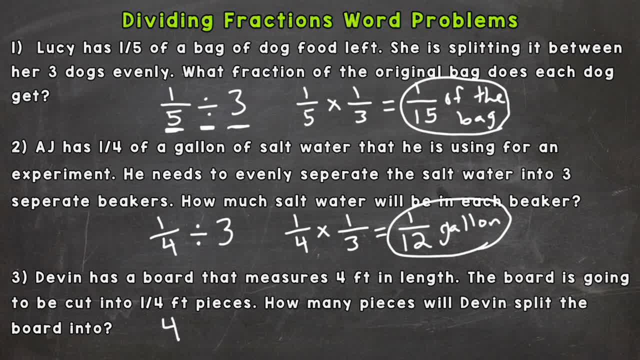 board. so that comes first: the 4 feet divided into groups of a fourth. so we're going to divide that 4 feet into groups of a fourth. so we're going to split that 4 feet into groups of a fourth. so 4 divided by a 4th, keep switch. 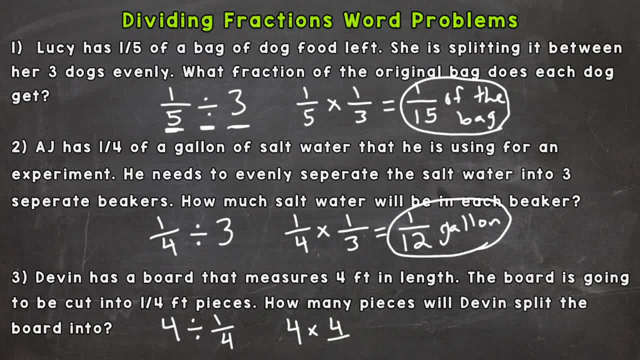 and flip and both of these whole numbers we can put over 1. so we have a top and a bottom. 4 times 4 is 16, 1 times 1 is 1, which 16 over 1 is just a whole 16. so 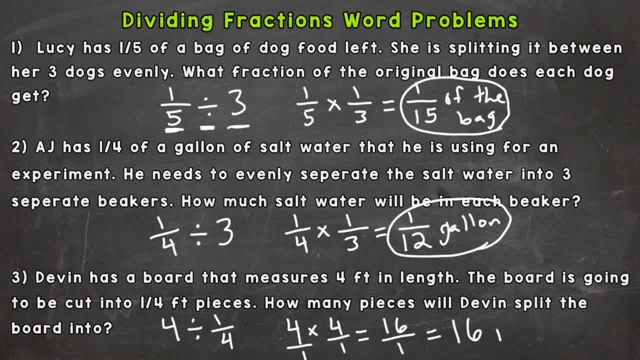 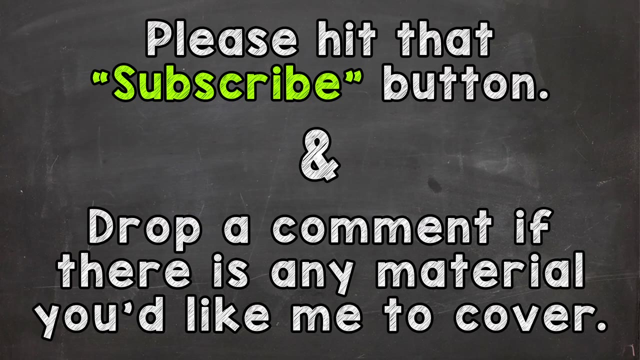 how many pieces will Devon split the board into? well, 16 pieces. so there you have it. there's a few examples of dividing fractions word problems. whenever you're separating or splitting into groups, you will use division. thanks so much for watching. until next time, peace. 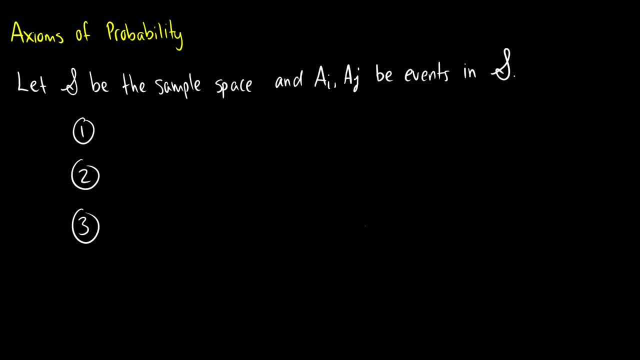 In this video we're going to talk about the axioms of probability. These are three crucial axioms that make up all the theoretical work and theorems that we have in probability. So here we go. Let s be the sample space, and a, i, a, j be events in s, so there can be an infinite amount. 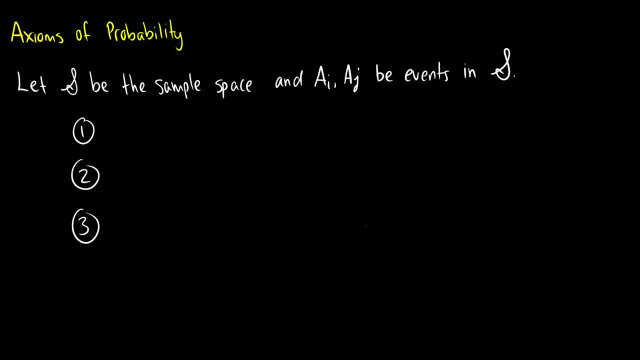 of them. Now, there's three axioms. One is that the probability of any event happening is going to be equal to or greater than zero. meaning we can't have a negative probability, which makes sense, because you can't say there's a negative 15% chance of something happening. You just say: 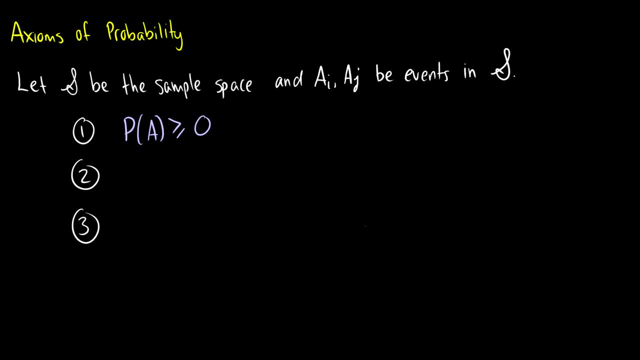 there's a 0% chance if it's not possible. The second axiom is that the probability of the sample space happening is going to be 1, which correlates to being 100% chance that if something happens, it's in the realm of all possibility. 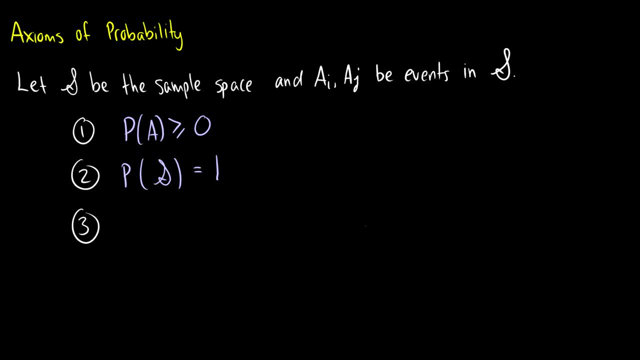 So if you flip a coin you can't have a 7 show up. It doesn't make any sense. The third one is a little bit more complicated. I'm going to show you the general form that would be taught in a statistics course and then break it down. So what this says is that if the intersection of all 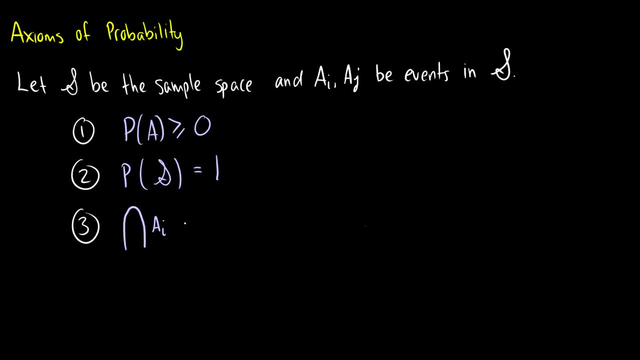 events is equal to the empty set, then the probability of the sample space happening is going to be equal to 0. So if you flip a coin you can't have a 7 show up. It doesn't make any sense. The third one is a little bit more complicated.